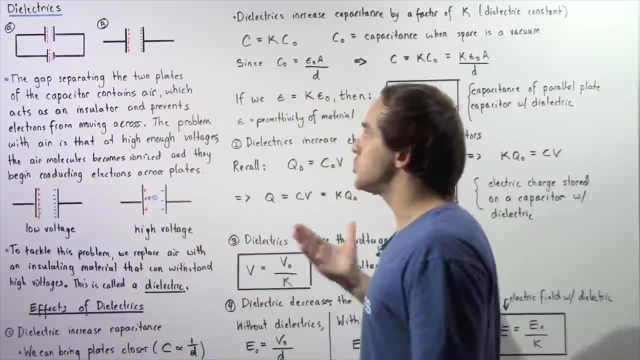 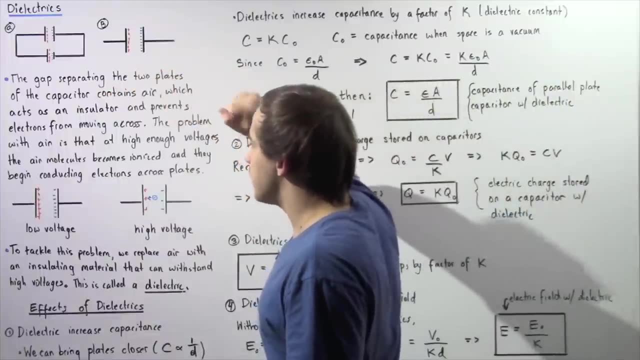 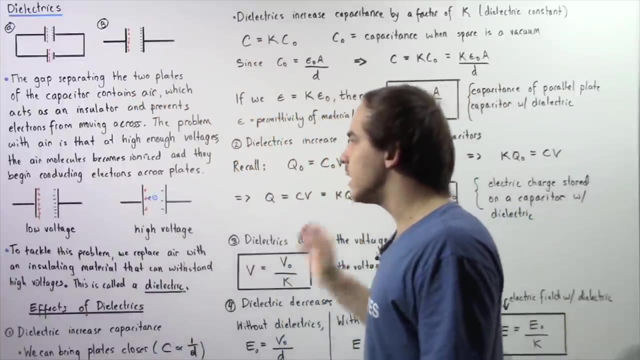 And we essentially have a loss of separation of charge and that destroys our capacitor. So once again, the problem with using air is that at high enough voltages the air molecules become ionized and they begin to disperse And they begin conducting electrons across the plate. 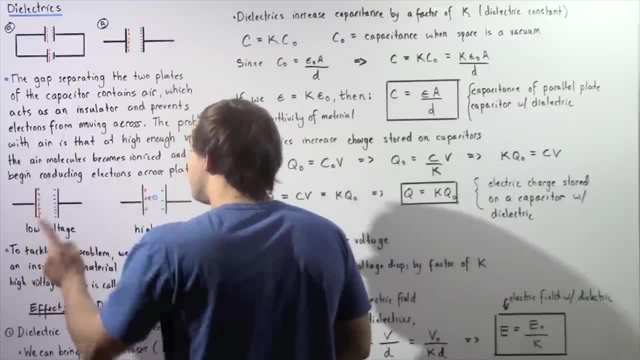 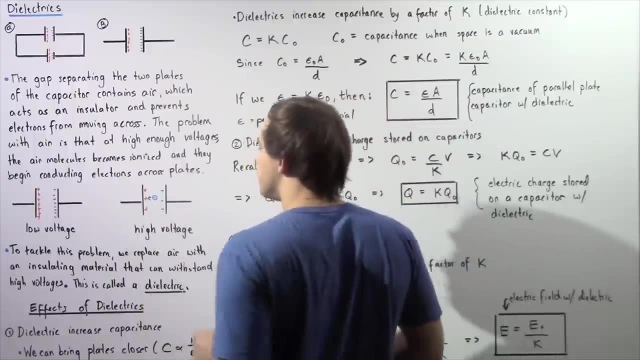 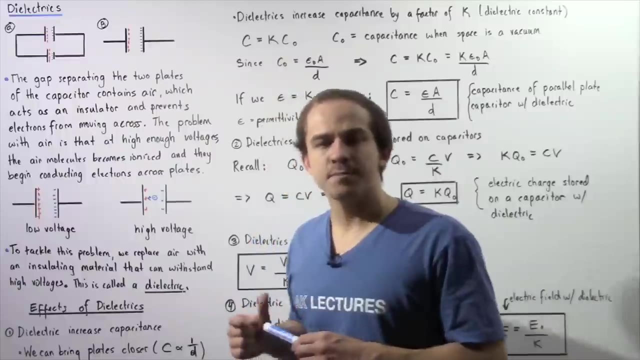 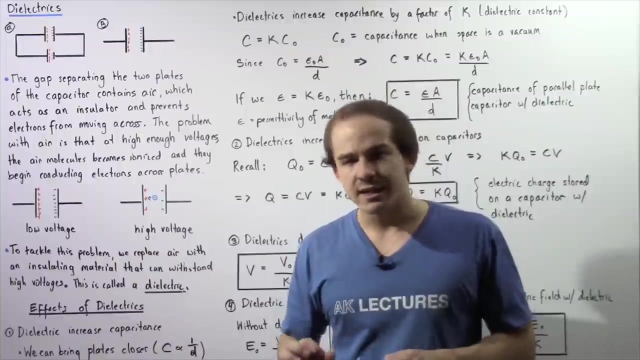 So at low voltages the air is a good insulator, but at high voltages it becomes ionized and allows electrons to flow from this plate to this plate, destroying our capacitor. Now, one way that we can tackle this problem is by replacing air with another type of insulating material that is capable of withstanding high voltages. Now, one way that we can tackle this problem is by replacing air with another type of insulating material that is capable of withstanding high voltages. Now, one way that we can tackle this problem is by replacing air with another type of insulating material that is capable of withstanding high voltages. Now, one way that we can tackle this problem is by replacing air with another type of insulating material that is capable of withstanding high voltages. Now, one way that we can tackle this problem is by replacing air with another type of insulating material that is capable of withstanding high voltages. Now, one way that we can tackle this problem is by replacing air with another type of insulating material that is capable of withstanding high voltages. Now, one way that we can tackle this problem is by replacing air with another type of insulating material that is capable of withstanding high voltages. 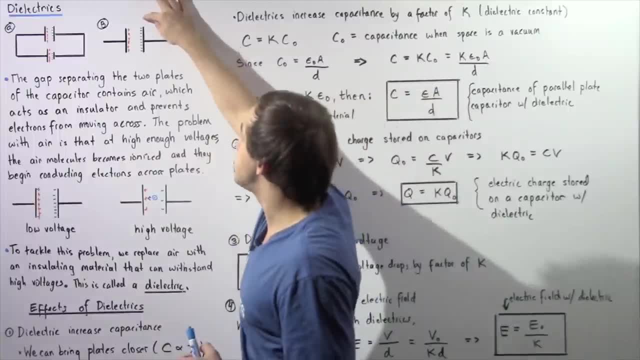 Now, one way that we can tackle this problem is by replacing air with another type of insulating material that is capable of withstanding high voltages- a dielectric. So we can place some type of dielectric in between our two plates. Now let's 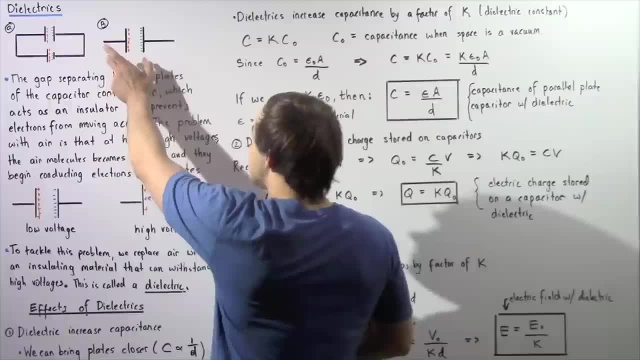 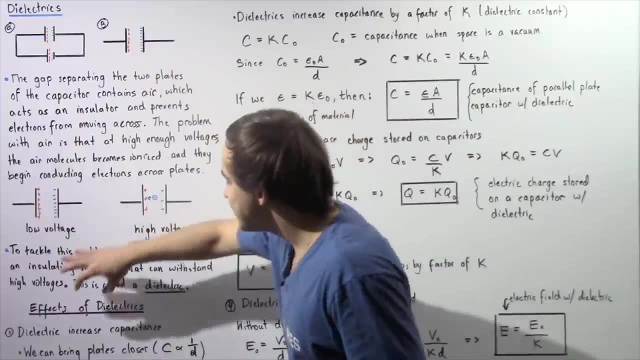 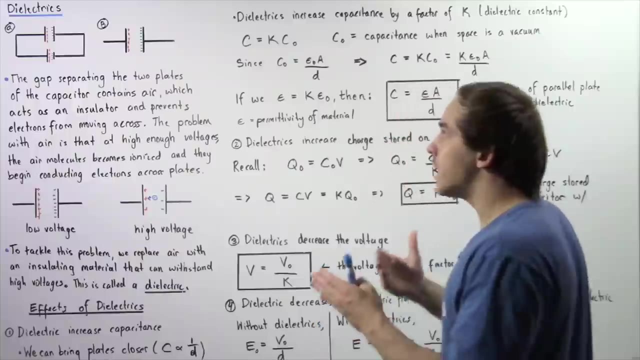 examine what the effects are of placing a dielectric between our two plates. So one thing that a dielectric does to a capacitor is it increases the capacitance, It increases the quantity of electric charge that can be stored on either one of our plates. So there are two ways. 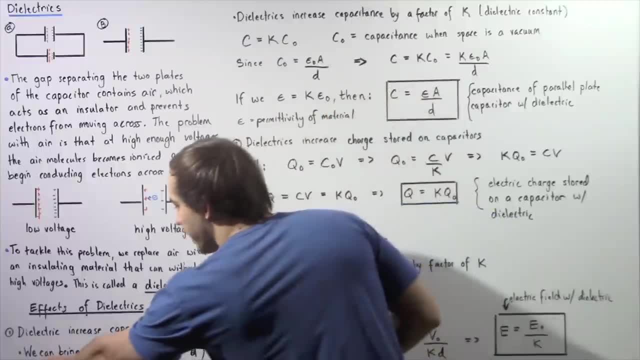 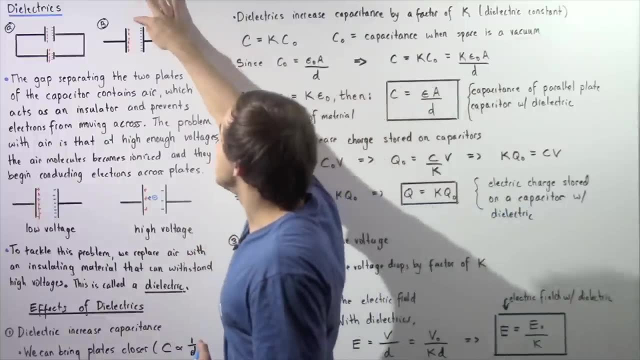 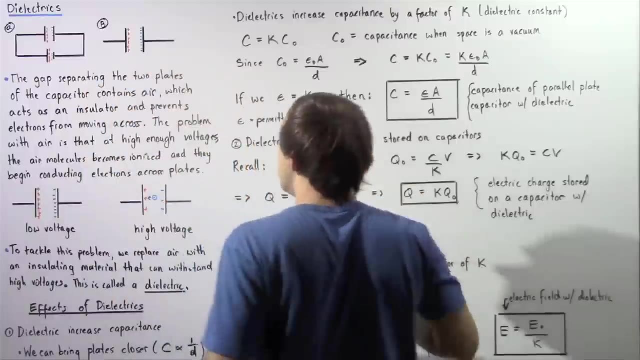 that we can increase our capacitance. So one way is we can bring our plates closer. So now that we have a very thin sheet of dielectric between our two plates, we can bring our plates closer, thereby decreasing our distance between our two plates, Because our capacitance is inversely. 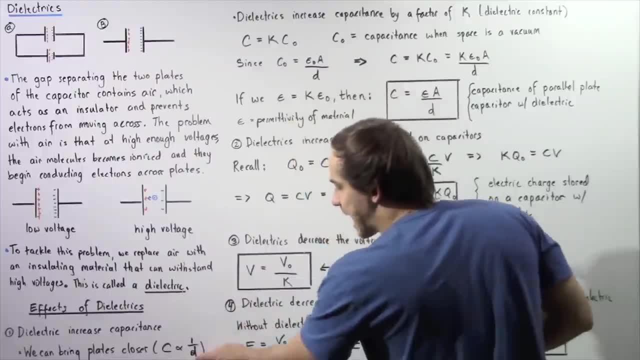 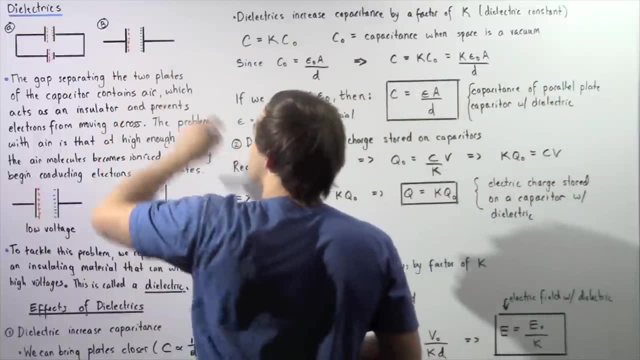 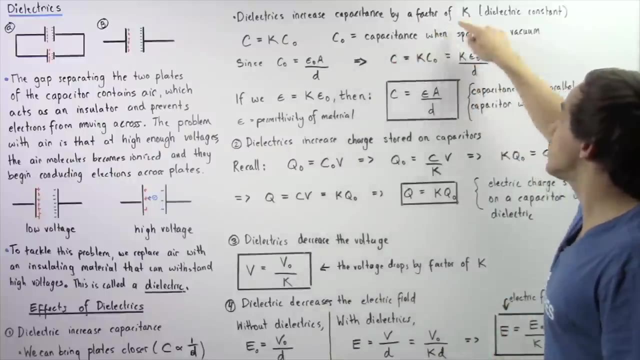 proportional to our distance. if we decrease our distance, we increase our capacitance. Now, even if our distance between the two plates remains the same, the dielectrics will still increase our capacitance by a factor of k, which is usually determined via experiment. Now, k is: 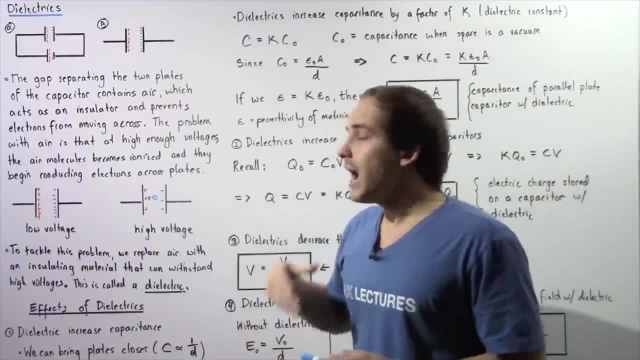 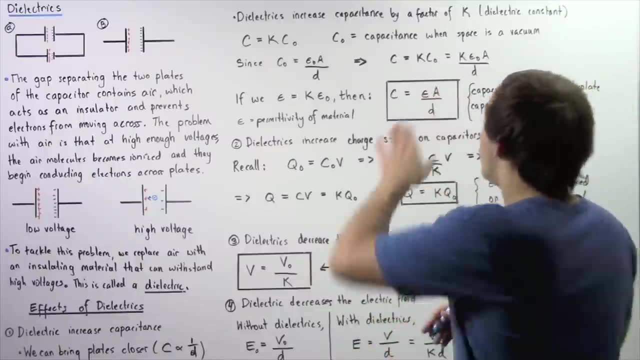 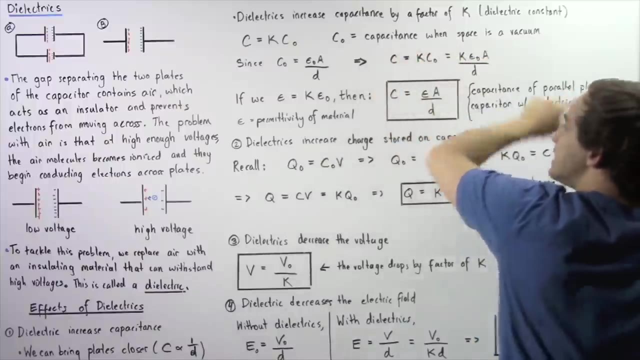 known as the dielectric constant, and it essentially depends on the type of substance that we are using, So different substances will have different k values. Now, what this basically means is the difference between a dielectric constant and a dielectric constant. So if we define our c0 as the 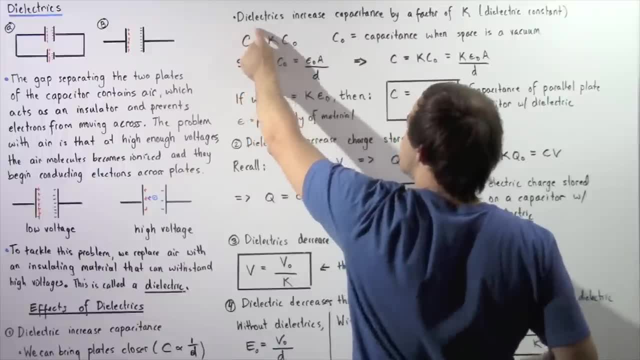 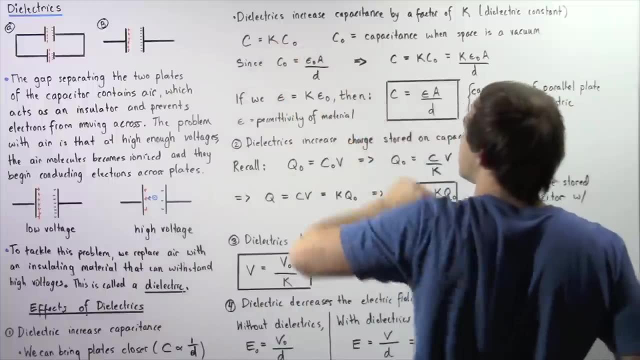 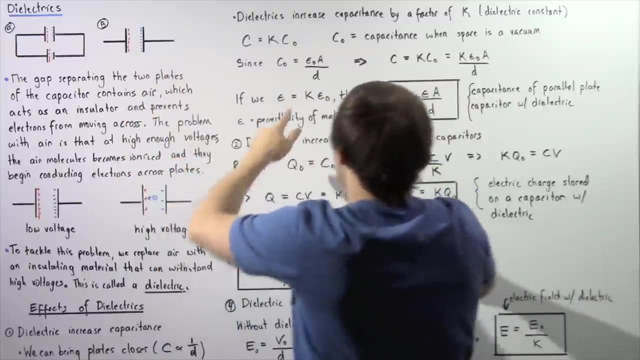 capacitance when the space in between our two plates is a vacuum. then we see that our capacitance c with our dielectric is equal to c0 multiplied by this factor of k. Now recall that c0, the capacitance when the space between is a vacuum, is equal to the product of the permittivity of free space. 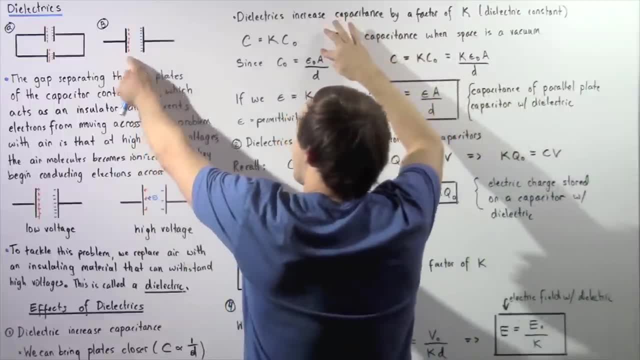 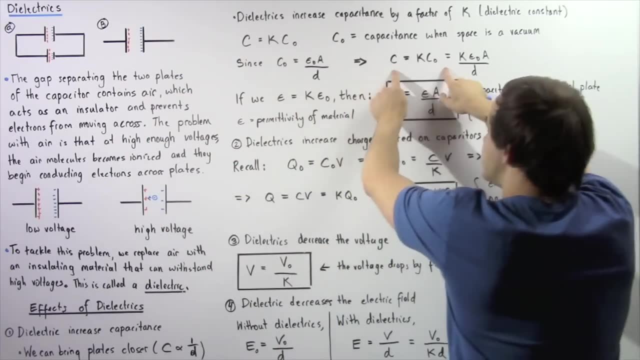 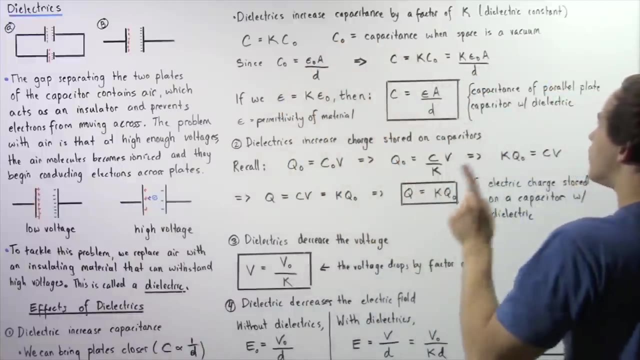 not multiplied by the surface area of either one of these plates, divided by the distance separating our two plates. So we can take this equation and replace c0 with this ratio and we get this result. So the capacitance with our dielectric is equal to the product of the dielectric constant k. 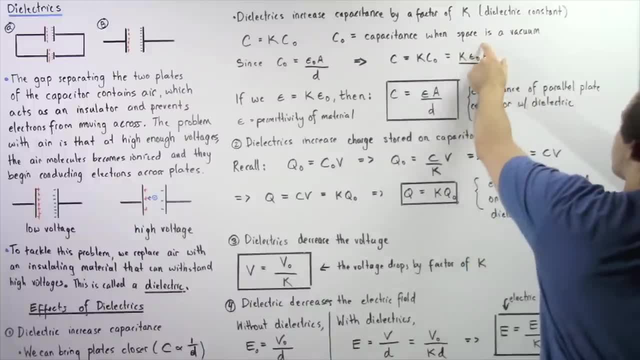 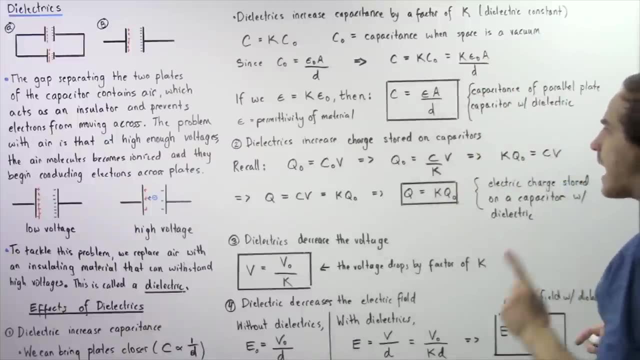 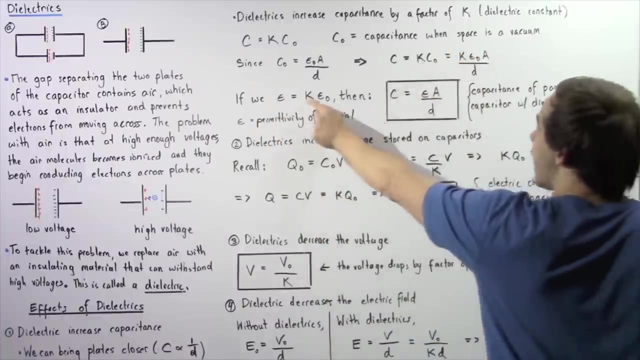 the permittivity of free space given by epsilon naught, the surface area of either one of the plates divided by the separation or the distance between our two plates. So if we now define a new constant given by epsilon to be the product of k and epsilon naught, then we have the following equation: So the capacitance of our 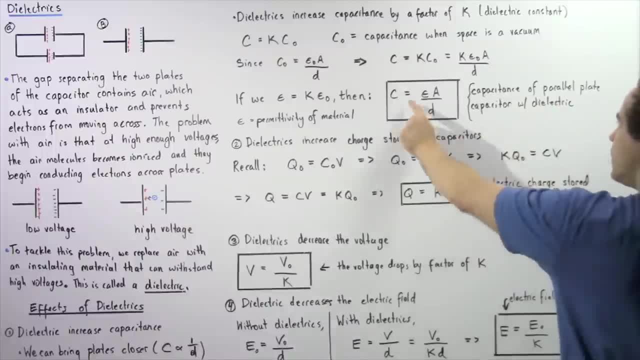 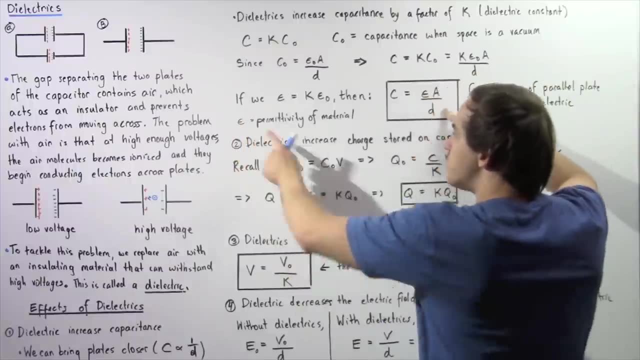 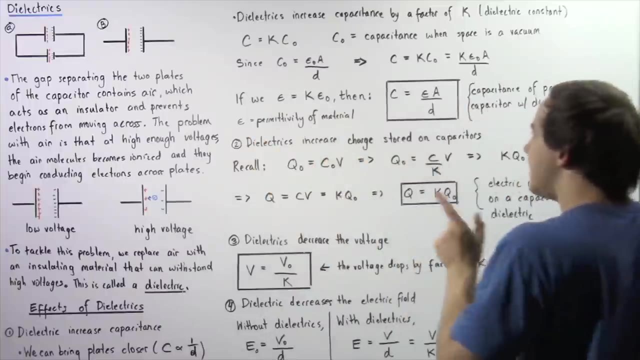 parallel plate capacitor with the dielectric in between, is equal to epsilon multiplied by a divided by d, where our epsilon is known as the permittivity of our dielectric constant. So if we now define a dielectric material that we are using, so once again epsilon is a constant. it's the product of the dielectric. 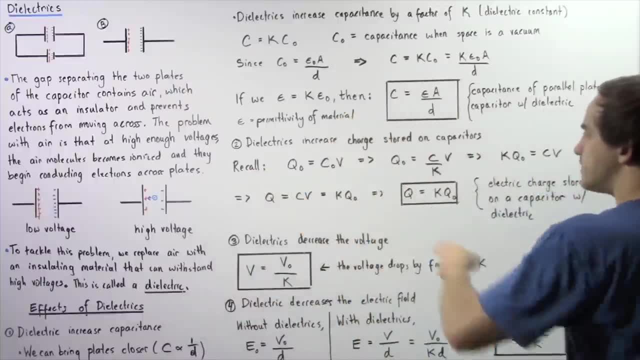 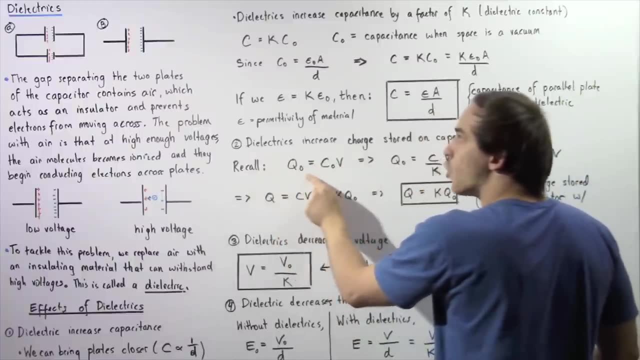 electrical energy. So if we now define a new constant, given by epsilon to be the product of dielectric charge, So let's see what that means by looking at the following equations. So recall that the quantity of electric charge that can be stored on our plate when there's a vacuum in between is equal to c naught. 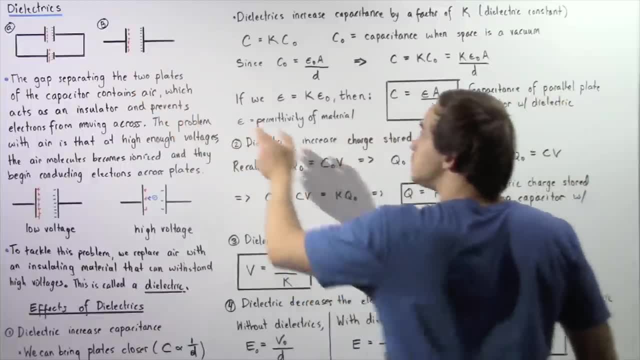 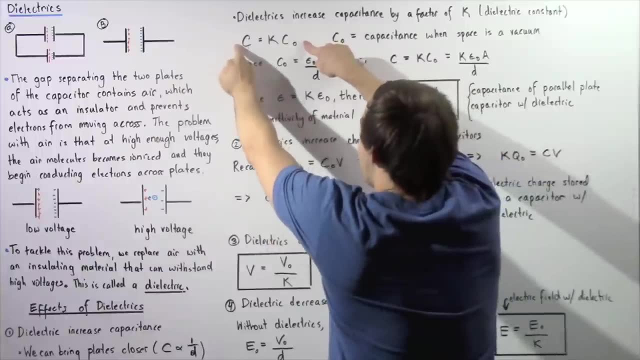 our capacitance when there's a vacuum in between, multiplied by the voltage difference. So q is equal to c multiplied by v. Now if we take this equation, rearrange it and solve for c naught, we can solve for the. 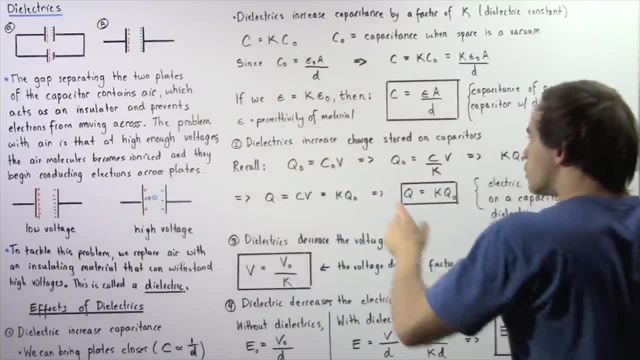 difference that we just came across, for We can see that c, naught, is equal to c divided by k. So let's replace c1 on 2za1, 0, 0, 0, 0, whereво c divided by k. So let's see, kids, how far is this momentum? 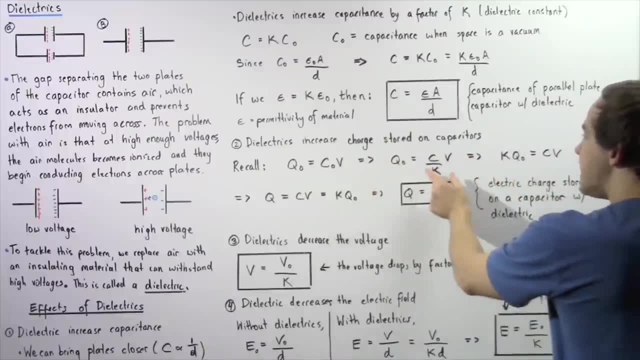 going? how far will the energyоту go? So let's return to the same equation. So somehow I can see that c0 is equal to c divided by k. So let's replace c0 with c divided by k. So now we have. 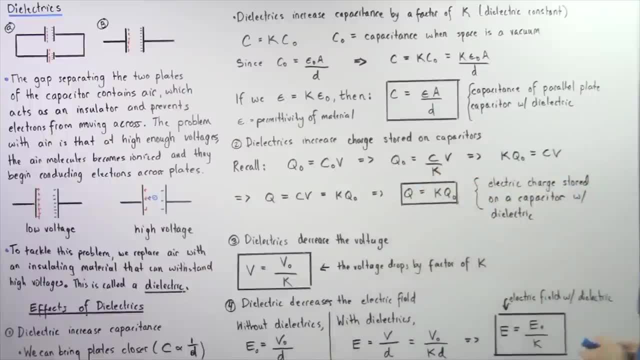 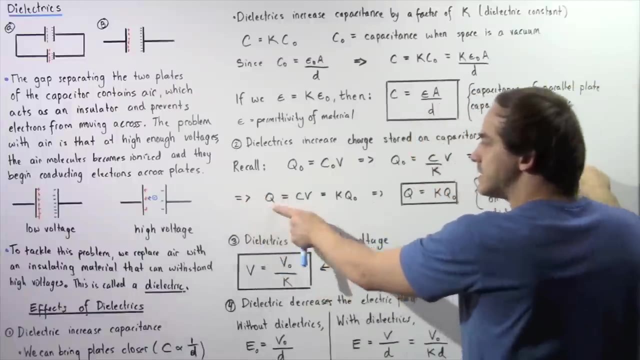 this equation. We can take k, bring it to this side, We get this result: the product of the capacitance of our dielectric capacitor multiplied by the voltage is equal to k multiplied by q. naught, So this is simply equal to q, the quantity of electric charge stored on our adolescent. Now, 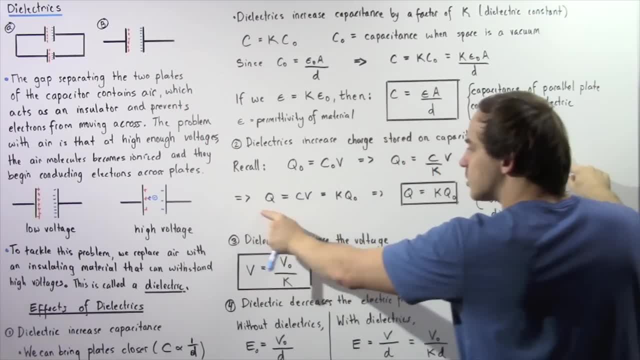 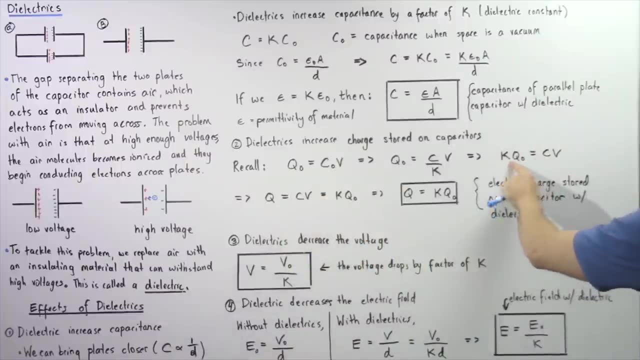 the next step. we get to this question here. The first thing we need to do here is to let us take charge stored on our capacitor when there is a dielectric in between. This is equal to Cv, which is equal to K multiplied by Q naught. So we see Q, the quantity of charge that is stored. 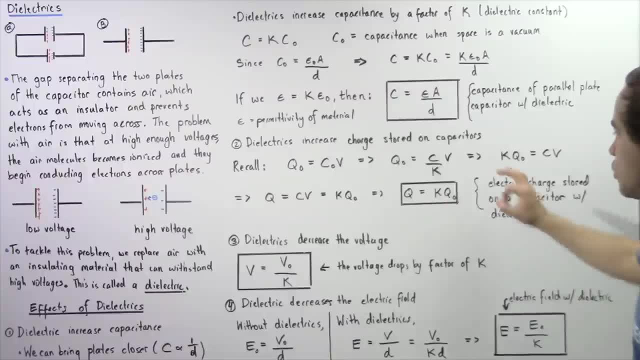 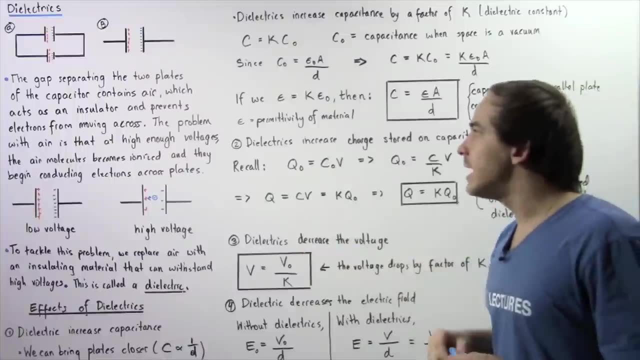 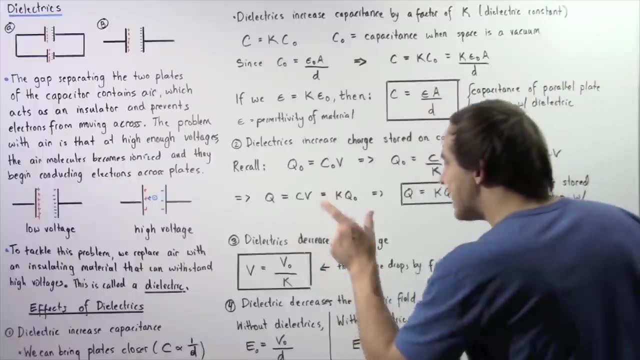 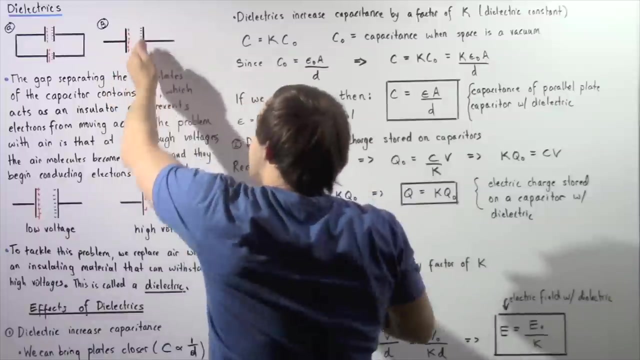 on our capacitor with a dielectric is equal to K, the dielectric constant multiplied by Q. naught, So let's move on to the third effect that our dielectric has on our parallel plate capacitor. So dielectrics decrease the voltage, So the voltage between our two plates when there's 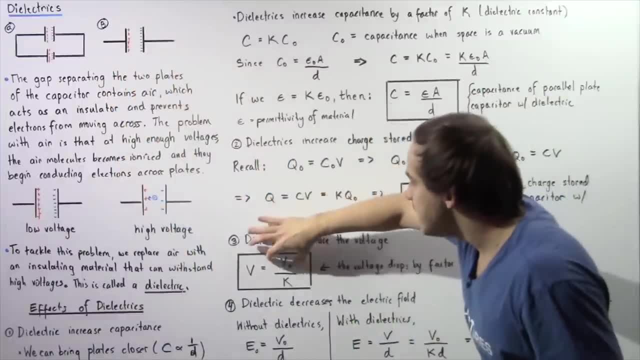 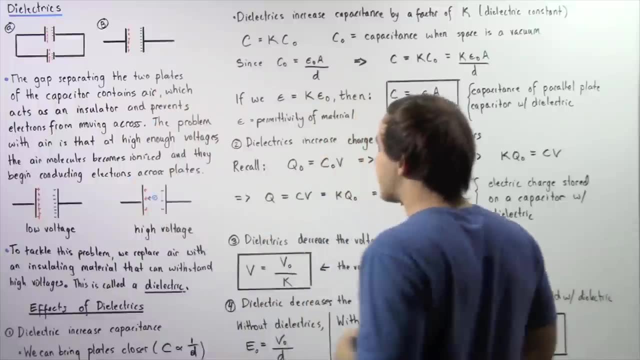 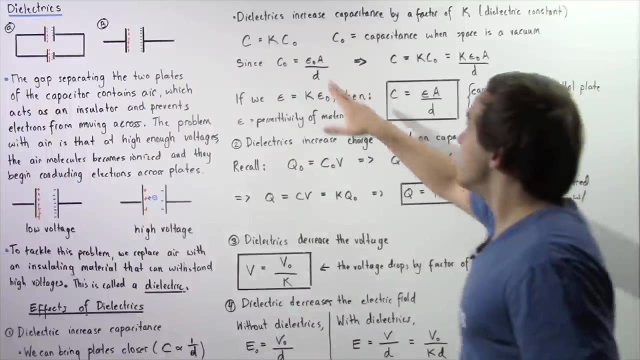 a dielectric in between is equal to V naught divided by K, where V naught is the voltage between our two plates when there's a vacuum in between. So we see, with the dielectric the voltage drops by a factor of K, So capacitance increases by a factor of K.